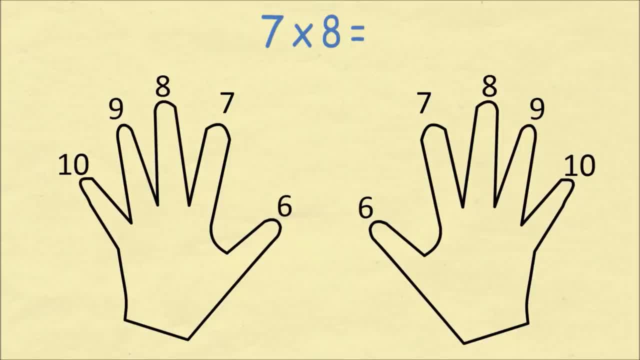 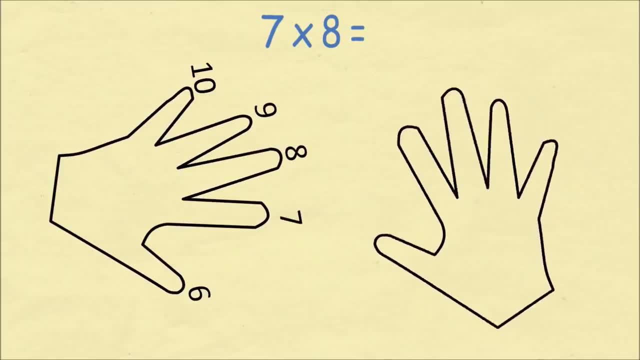 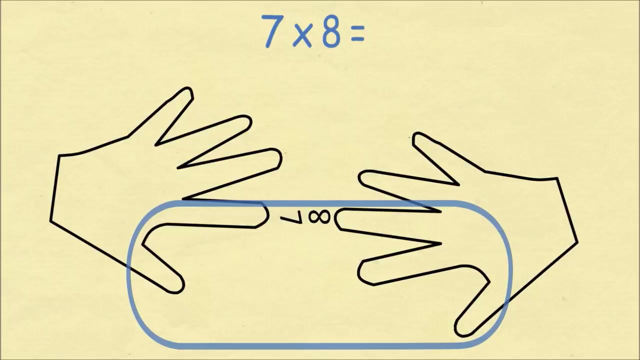 pinky finger. Let's do the problem of seven times eight. We'll rotate our left hand, so we have one finger being seven, and we'll rotate our right hand to line up the number eight. Now we'll count the numbers of fingers that are below the two fingers which are touching. We have two fingers on the. 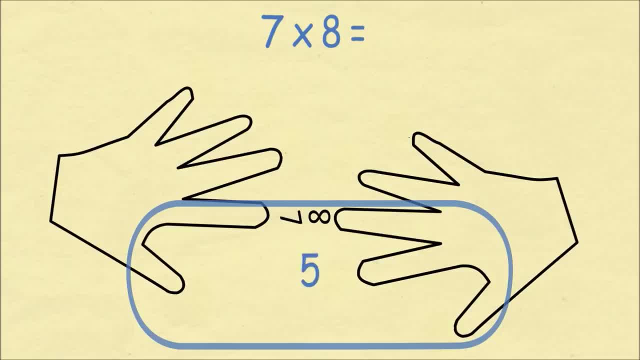 left hand and three fingers on the right hand, which is a total of five fingers. This becomes the tens digit of our answer. The fingers that are above the touching fingers are three on the left hand and two on the right hand. We'll rotate our right hand to line up the number eight. 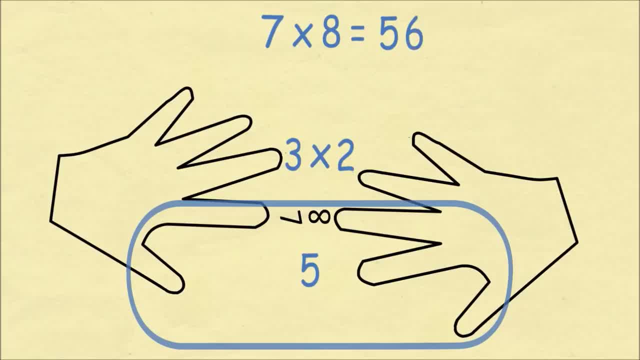 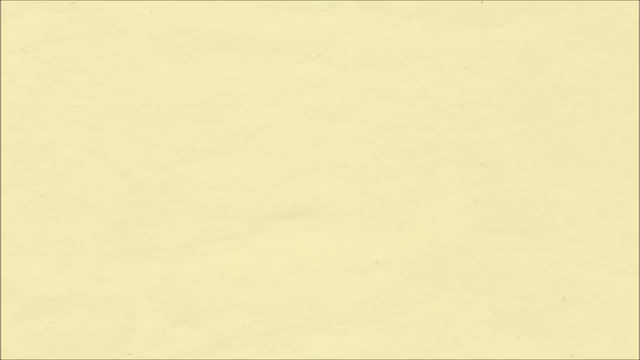 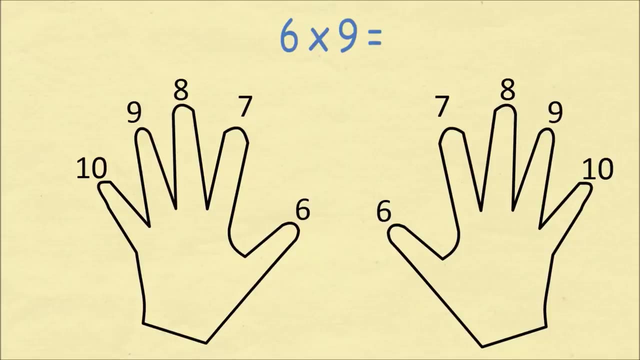 We multiply these Three times two is six and that gets us our answer of 56.. You can use this procedure anytime you're multiplying two numbers between six and ten. Let's do another example of six times nine. We'll rotate our left hand so that we are having 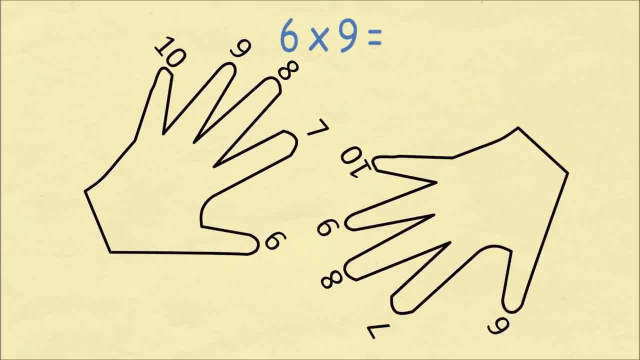 the number six and we're going to rotate our right hand to line up the number nine. We now count the hands and the dropped fingers. We'll again fold over our numbers five". Four and five are rainbows and purple arewords. Two and five are ribbons and purple areuffins". 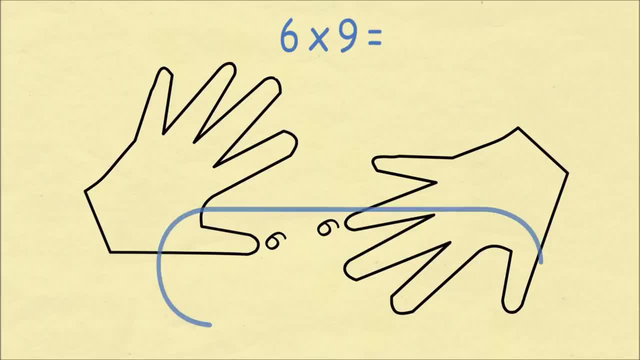 We're going to duplicate those to make a slipperyville in memory of the six. depending on how you're doing, We'll use our little blue and white fingers to make a slipperyville and then you'll put them to learn how to call them the number of fingers that are below the fingers that are touching, including the fingers that are 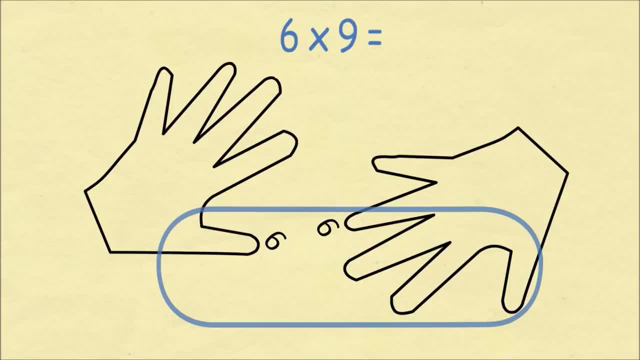 touching. So we have one finger on the left hand and four on the right hand, which becomes five fingers, and this is 50 because the fingers that are below the fingers that are touching are always counted as tens. Now we have four fingers above the fingers that are touching and one finger on 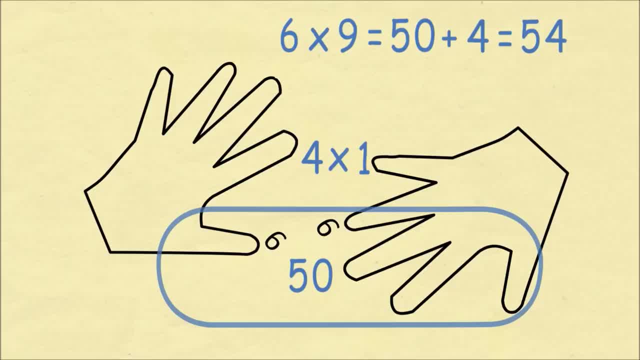 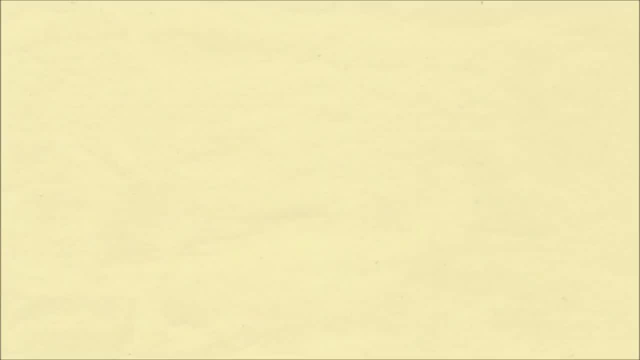 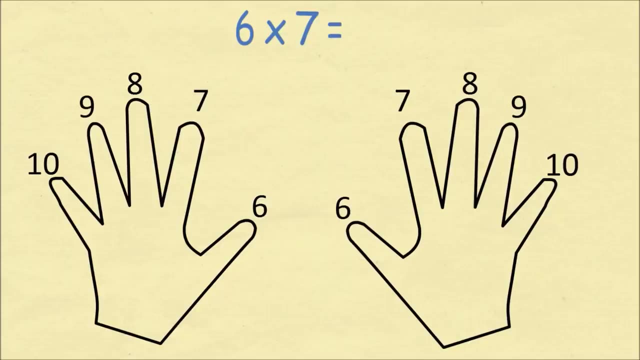 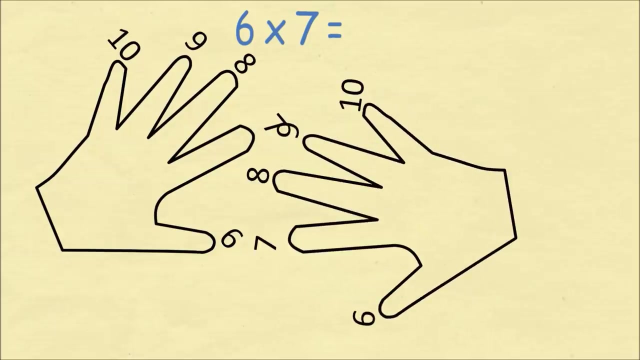 the right hand. We multiply these and we have four. We add those two numbers, 50 and 4, to get our answer of 54. This procedure always works for the numbers 6 through 10.. Let's do a final example of 6 times 7.. We'll rotate our left hand so we have the thumb as the finger. 6. We rotate our. 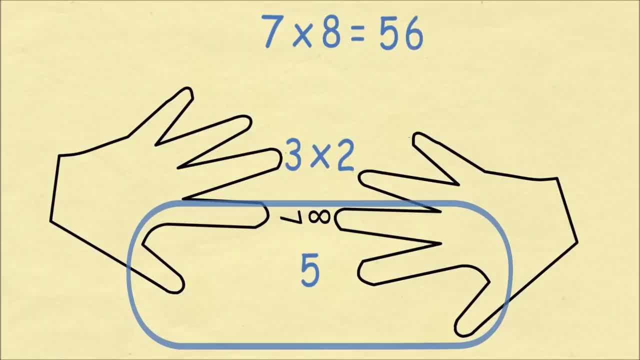 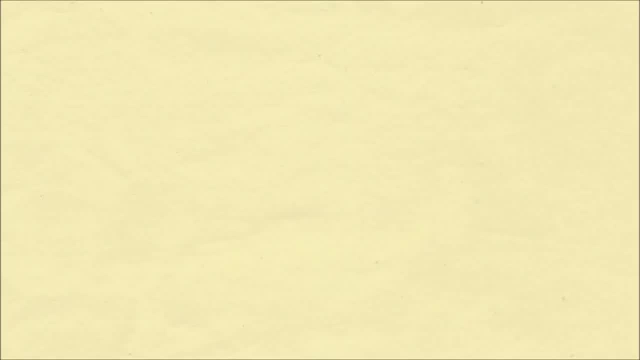 Now we'll count the numbers of fingers that are below the two fingers, three on the right hand. We multiply these three times two is six and that gets us our answer of 56.. You can use this procedure any time. you are multiplying two numbers between six and ten. 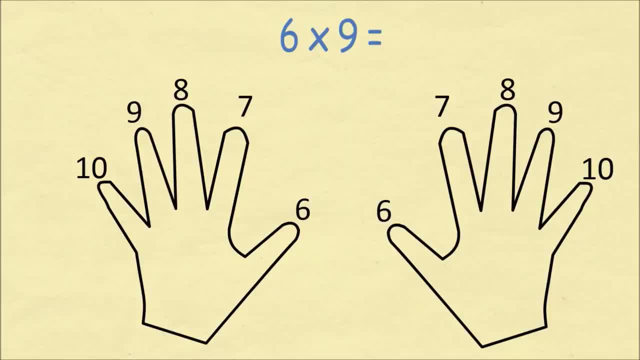 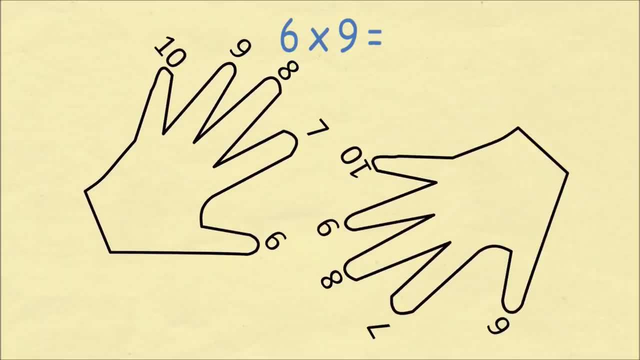 Let's do another example of six times nine. We'll rotate our left hand so that we are having the number six and we are going to rotate our right hand to line up the number nine. We now count the number of fingers that are below the two fingers in front of us. 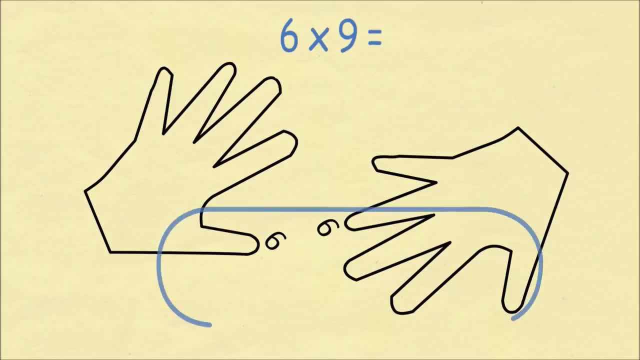 the number of fingers that are below the fingers that are touching, including the fingers that are touching. So we have one finger on the left hand and four on the right hand, which becomes five fingers, and this is 50, because the fingers that are below the fingers that are touching are always 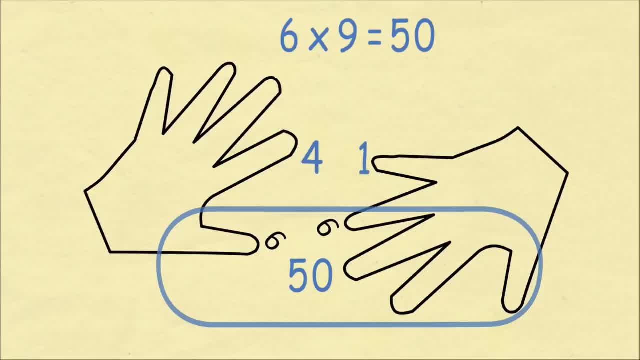 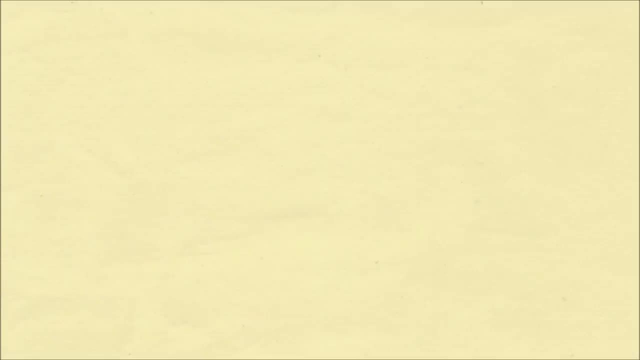 counted as tens. Now we have four fingers above the fingers that are touching and one finger on the right hand. We multiply these and we have four. We add those two numbers, 50 and 4, to get our answer of 54. This procedure always works for the numbers 6 through 10.. Let's do a final example. 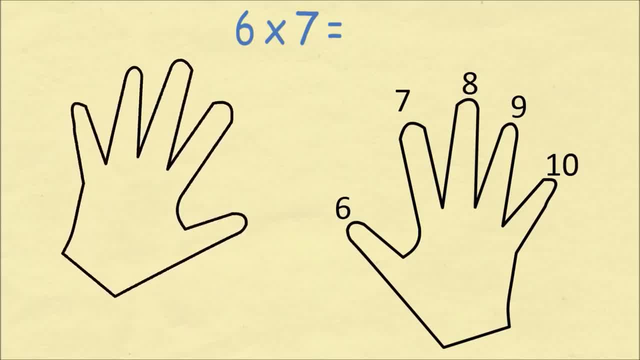 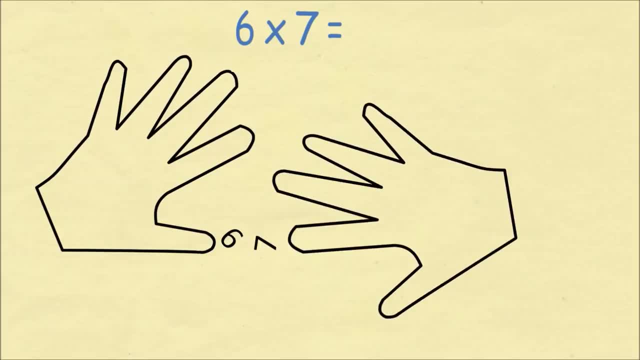 of 6 times 7.. We'll rotate our left hand so we have the thumb as the finger 6. We rotate our right hand to the index finger of 7.. Now we count the number of fingers that are below the fingers that are touching. including those two fingers, We have one on the left hand and two on the right. 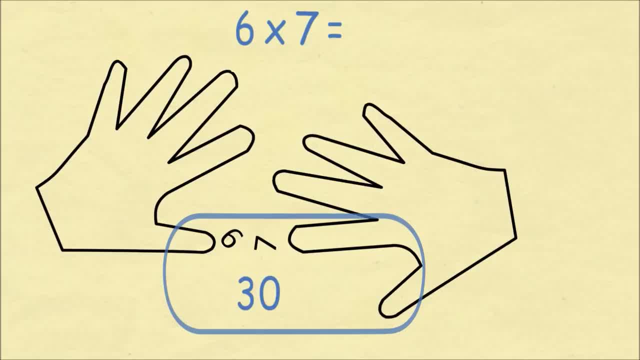 hand, which makes for 3 or 30. Now we count the fingers which are above the fingers which are touching. On the left hand we have 4, and on the right hand we have 3. We multiply these 4 times 3 is 12.. So we add 30 and 12 to get 42. And in fact we have a number of fingers that are below the. 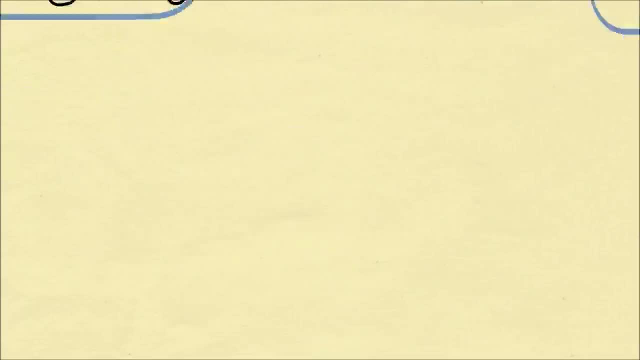 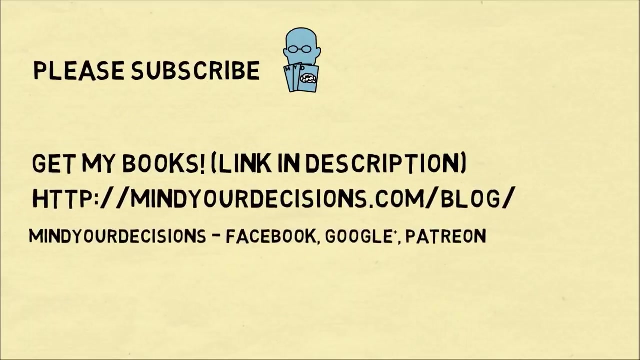 fingers that are touching. In fact, 6 times 7 is 42. So it's a pretty neat trick. Thanks for watching. Please subscribe to my channel. I make videos on math and game theory. You can get my books about math. There's a link in the video description. You can catch me on my blog. Mind Your Decisions.